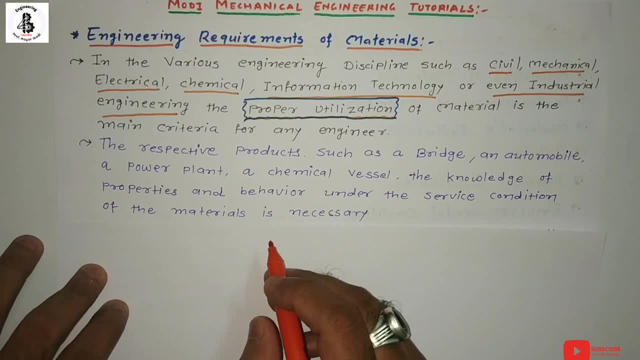 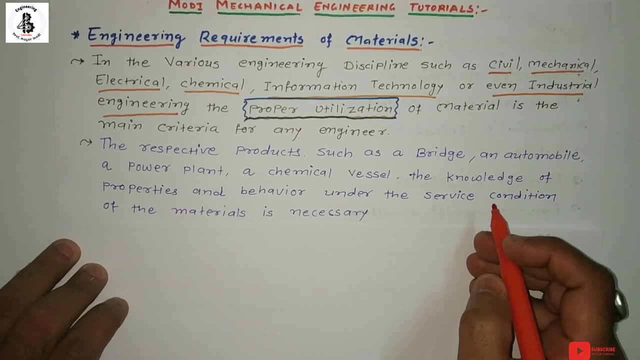 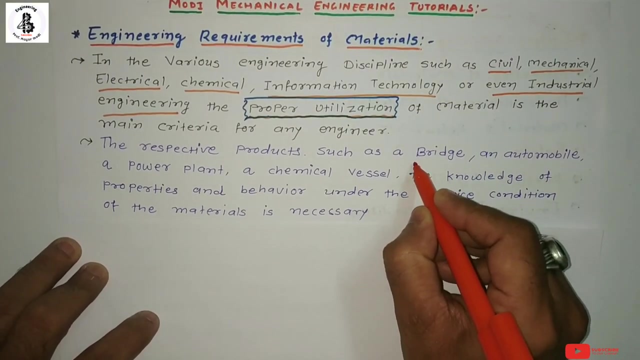 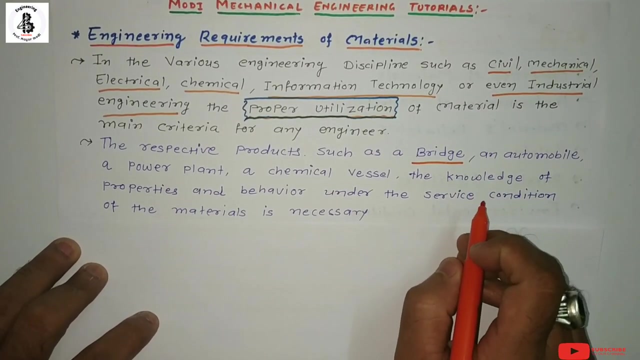 Why the customers? So in second topic, So basically the various kind of applications that will be correlated with the different branch of engineering, or you can say the discipline of engineering. So the respective products, such as bridges. So bridge is basically for the civil engineers. So according to my requirements and life of that particular bridge, We would select such kind of materials that will be having a 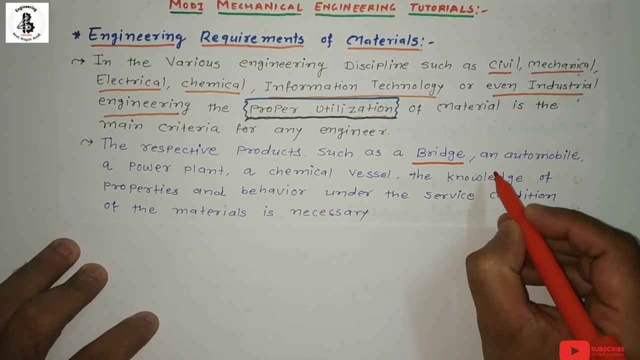 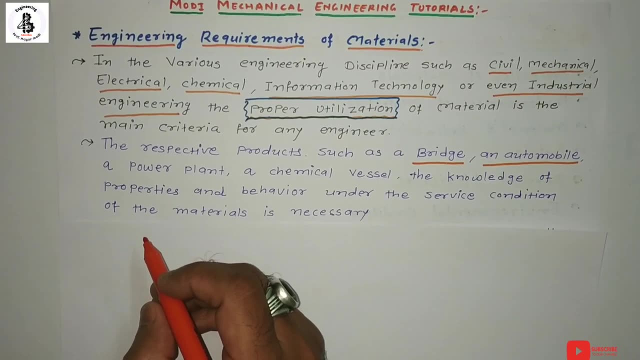 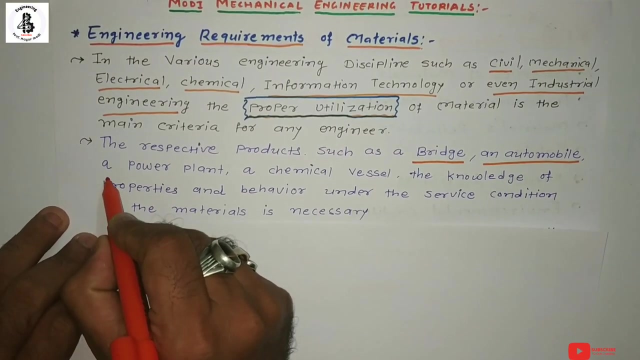 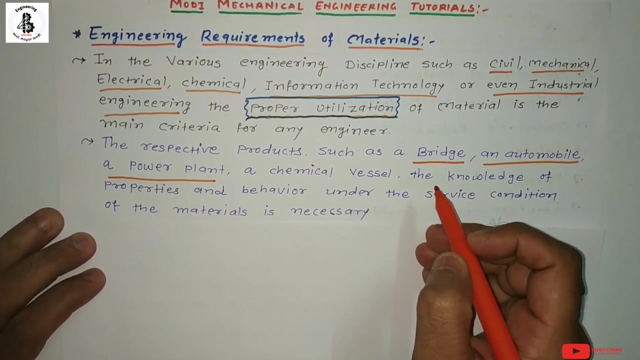 good Performance, then second applications, like an automobile. So basically, according to my requirement of the weight, then the performance of the products and durability, we would like to select over materials. Then power plants, generally power plants. It will be used to developing electricity, So that would be of very high temperature applications. 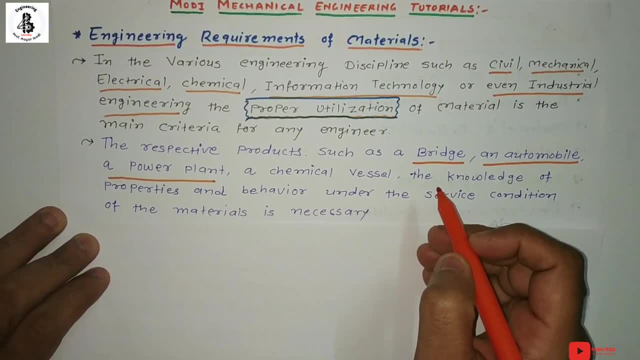 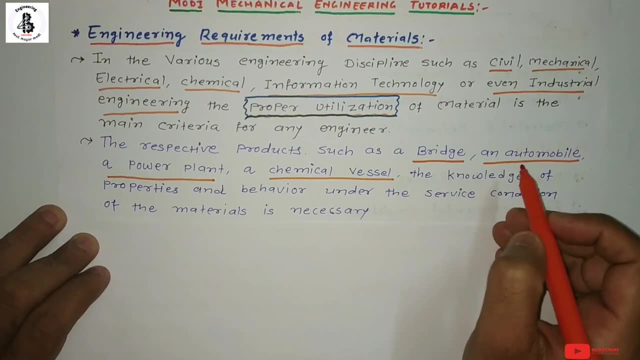 So all the components that are only developing electricity. It will be having that high temperature applications The power plants will have a power矛 swollen would be have Lenlo动 shi depends upon the high temperature applications than chemical vessels. so in the case of chemical, 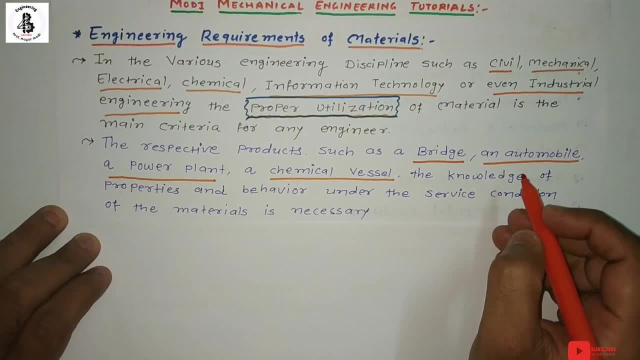 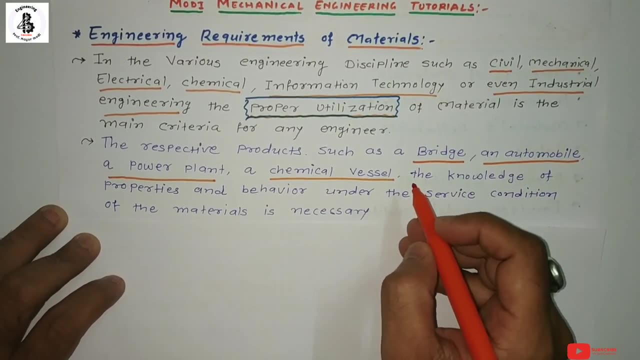 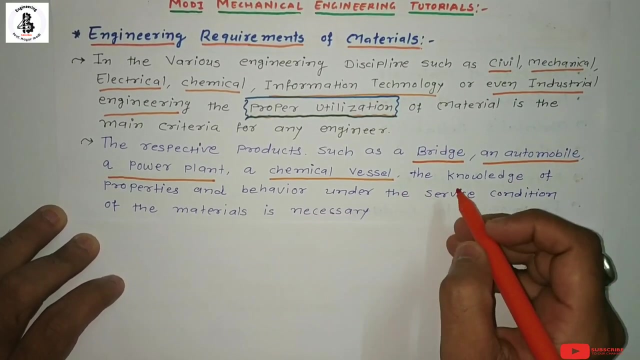 industries, storage as well as transportation of the one chemical from one place to another place. so we would like to select such kind of material that will be not chemically affected by the environment or not that material. it will be affected by the any kind of materials. so the 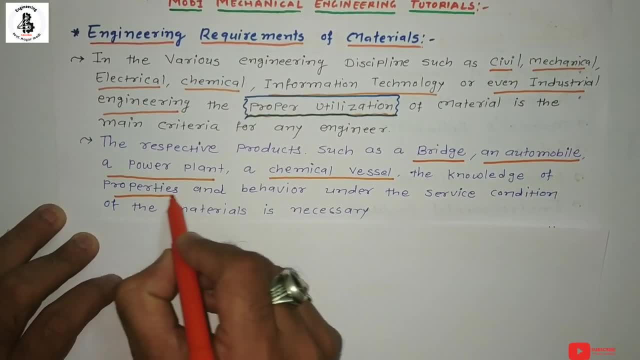 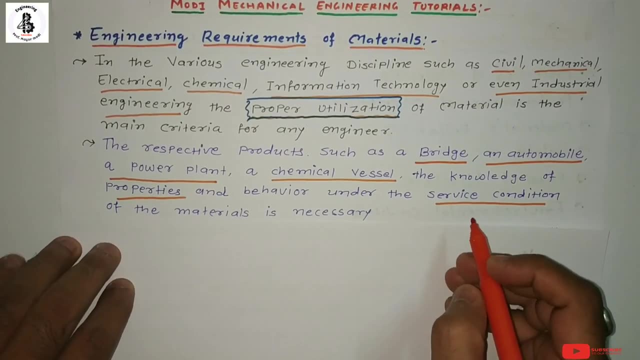 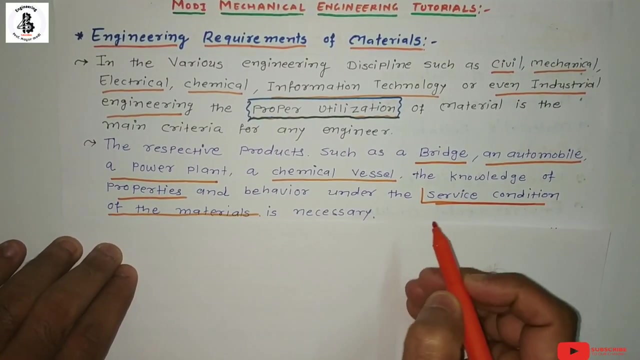 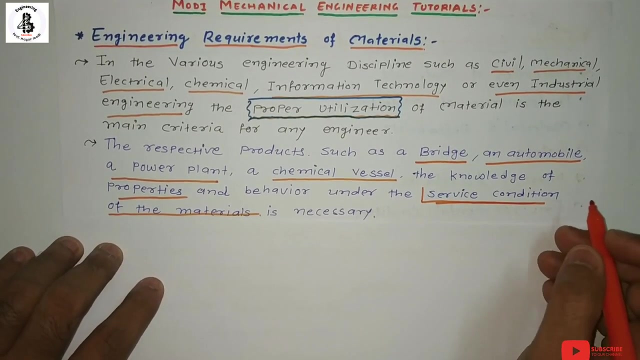 basic knowledge of that particular properties and behavior under the service condition of the materials. so in second topic more focus only on to the service condition of the materials is necessary so that service condition it will be like under the loading condition of the materials, so different applications it will be having a different conditions, if i am talking. 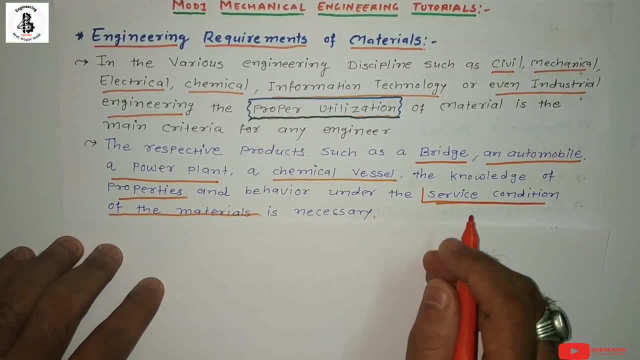 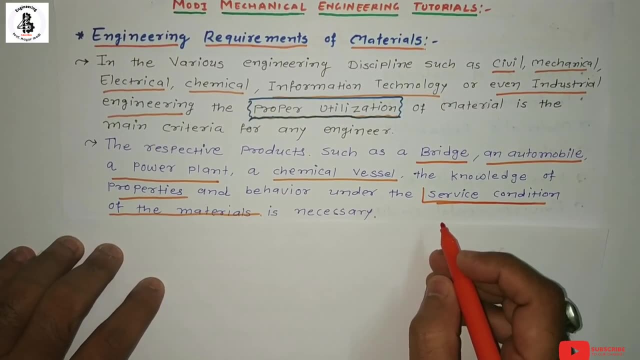 about boilers and other materials, then it will be like, under the loading condition of the materials, so boiler, that will be the high pressure, high temperature applications, so that selected material it will be with staining at higher temperature, as well as your higher pressure, some bridge materials, so it will be having a different environment conditions for automobiles. 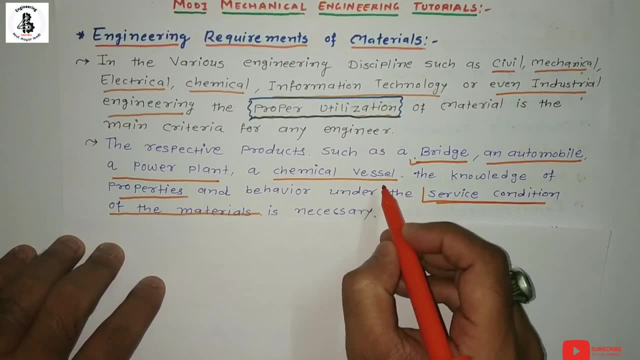 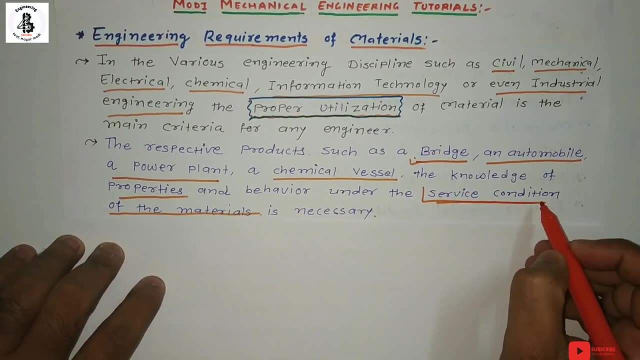 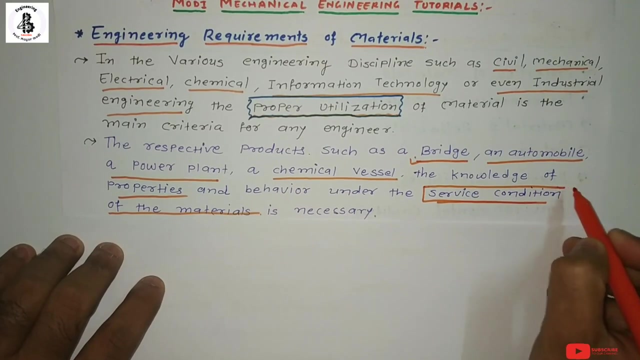 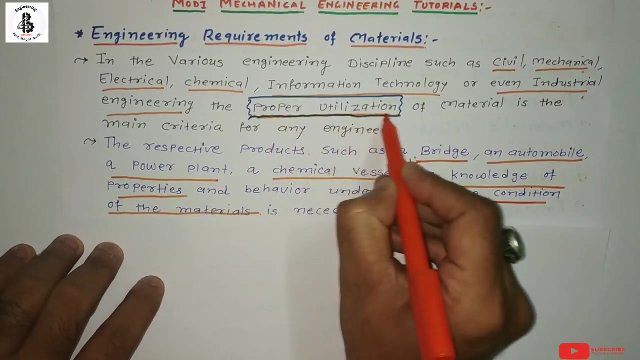 different conditions for chemical vessels. it will be different conditions so you have to examine, or you have some basic knowledge about that- service conditions or you can see that under the loading conditions. so second part, that will be related with the service conditions or under the loading conditions, and that conditions it will be having a proper utilization of the selected materials. so 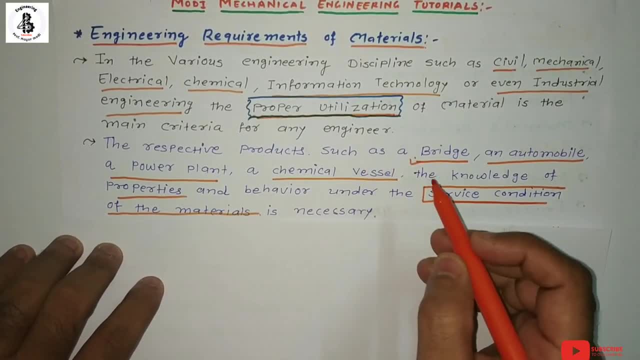 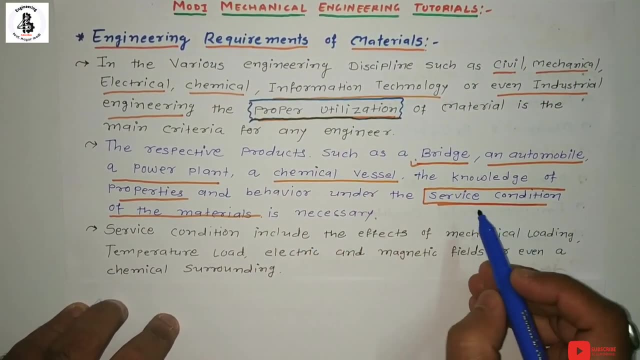 that too, it will be the basic engineering requirements of the materials. in third section, as we already discussing, into the proper utilization of the selected material, into the under the loading conditions, or you can say the service condition of the materials, so that service conditions that will be including the mechanical loadings. so mechanical loading, that 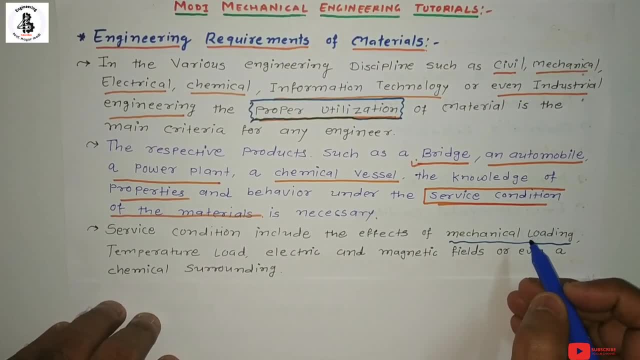 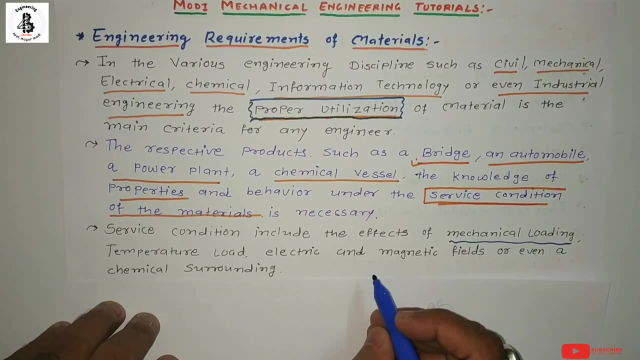 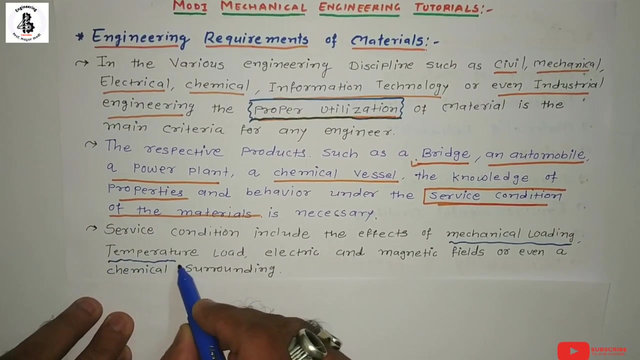 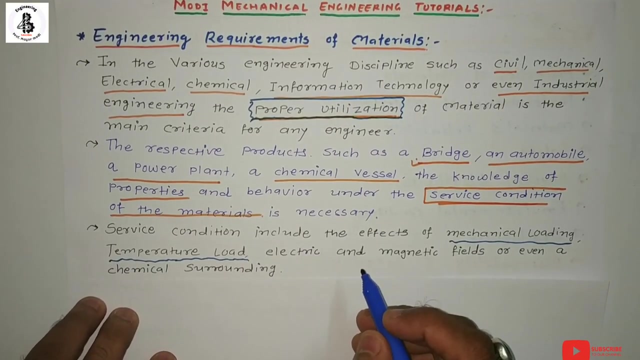 will be repeated loading, or you can say fatigue loading, tensile loading, compression loading, so any kind of that loading it will be considering as a mechanical loading. then temperature, so temperature having a vital role for changing their properties of the any kind of materials, so all the materials, or you can say metallic materials, it will be having a higher temperature. 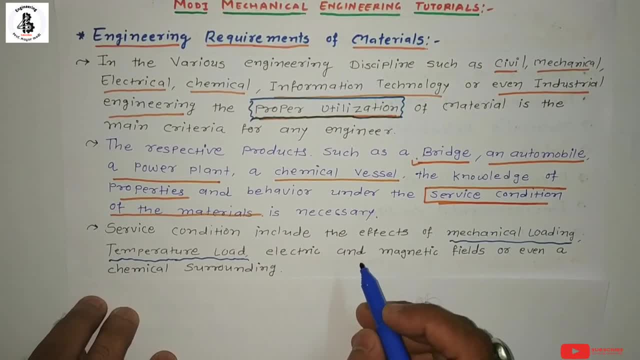 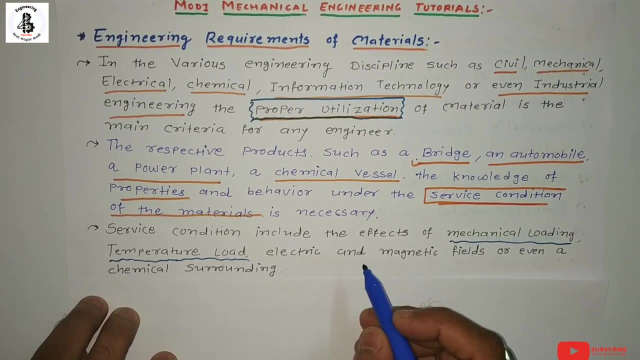 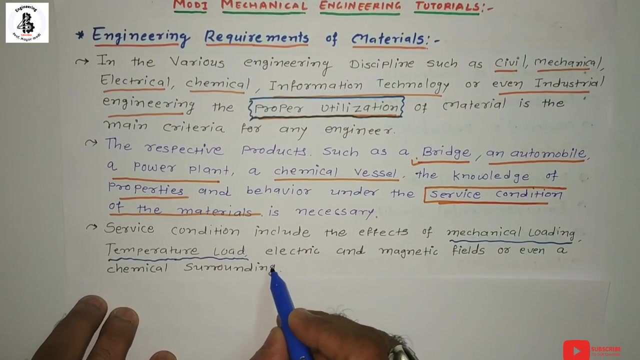 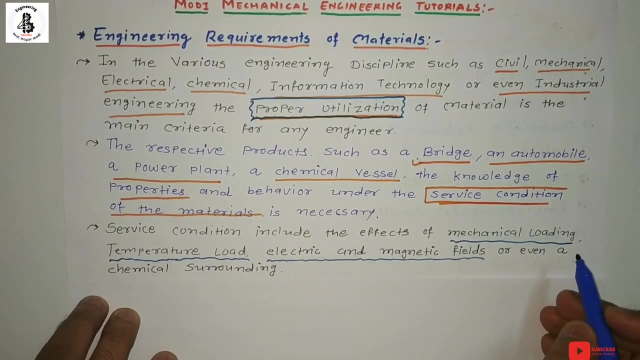 it will be changes the properties and its property is going to be changed. so it structure is change and according to structure is change, its behavior it will be change. so second important part for the service condition, that will be included as a temperature. then electric and magnetic fields, say, if you work on to the any kind of conductive materials for transferring the 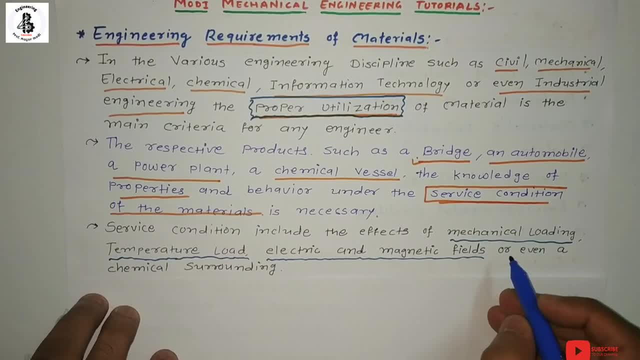 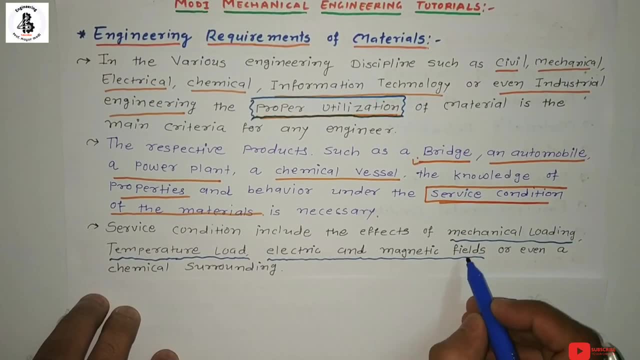 electricity from one place to another place. so in that case- you can see that there are a lot of case- it will be the generation of the magnetic field, So that magnetic field that will be affected any other neighborhood materials, So such kind of material it will be having a 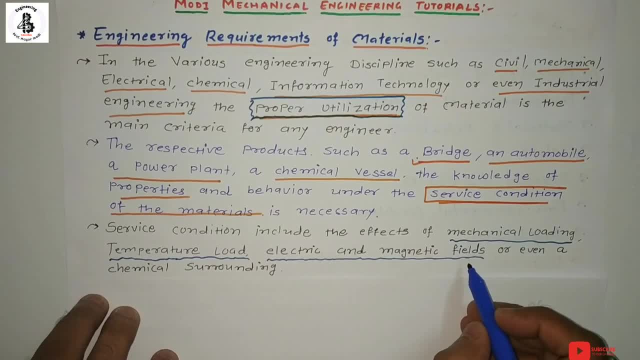 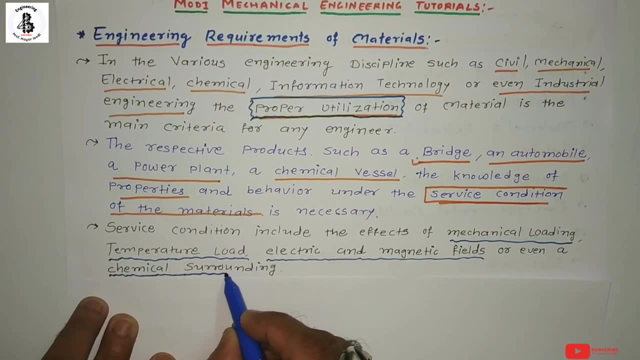 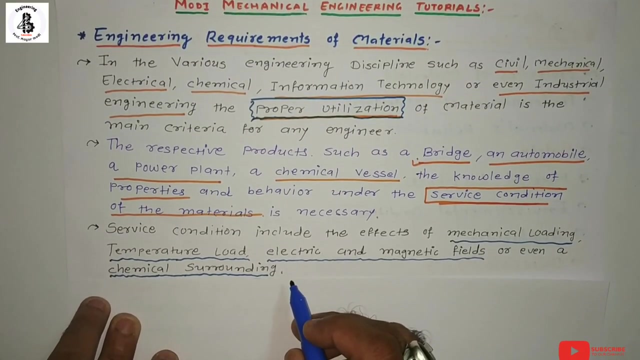 restraining such kind of magnetic fields or you can say chemical surroundings. So by the in contact of the chemical, all the materials, that will be deteriorating the properties of the metals, So our selected material, it will be restraining all that characteristics at that chemical surroundings, Suppose. I want to taking one example of the food industries So that 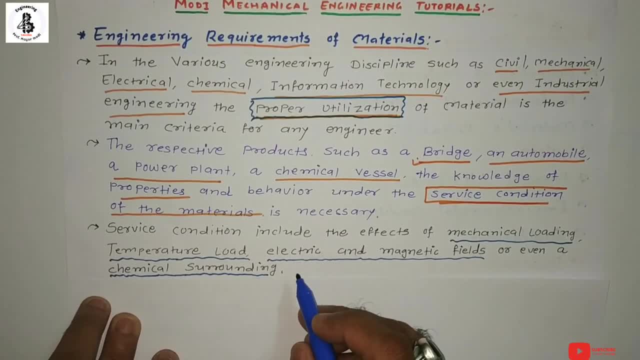 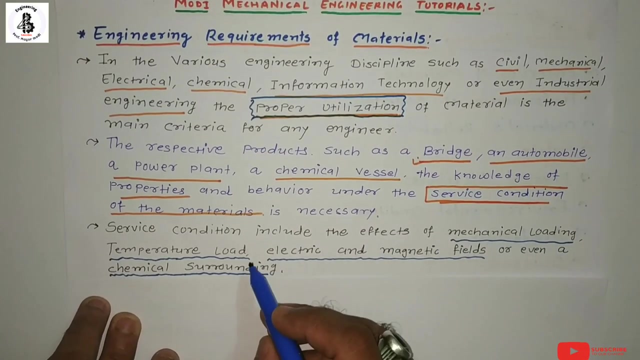 storage of the food as well as the processing onto the food. it never reacts with the. any kind of component is being used for the production of the foods. So that will be the one kind of examples. So the service conditions: It may be mechanical, it may be temperature load, electrical load, magnetic load, or you can say 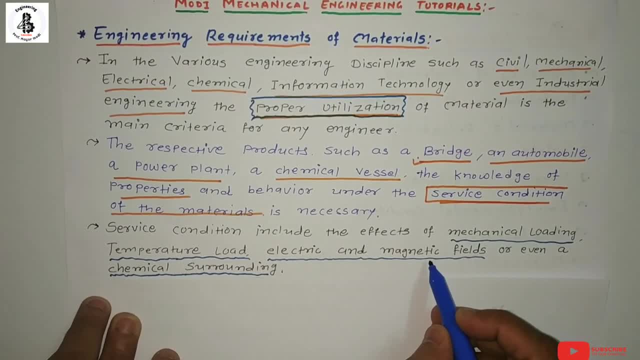 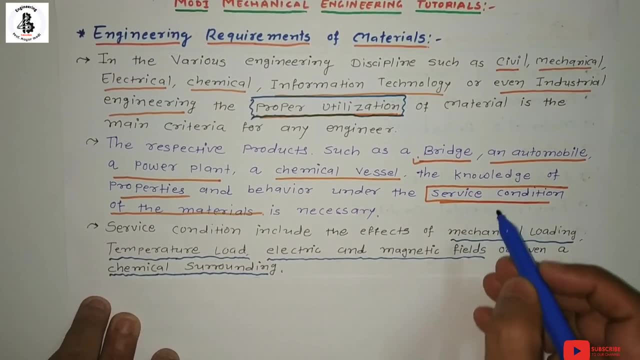 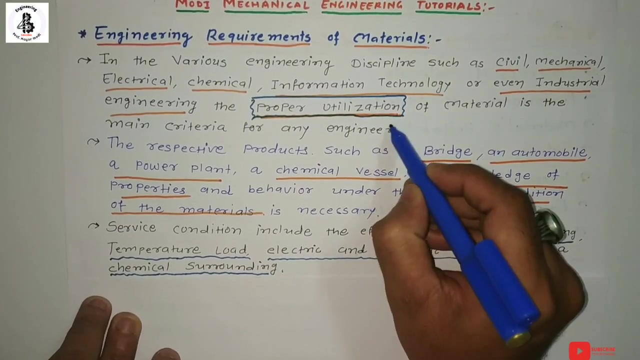 environment conditions. So these all are considering as a loading. So you can say service loading or you can say that under the loading conditions, So that loading conditions it will be having a proper utilization of the materials. So these three are the main proper utilization. Second, 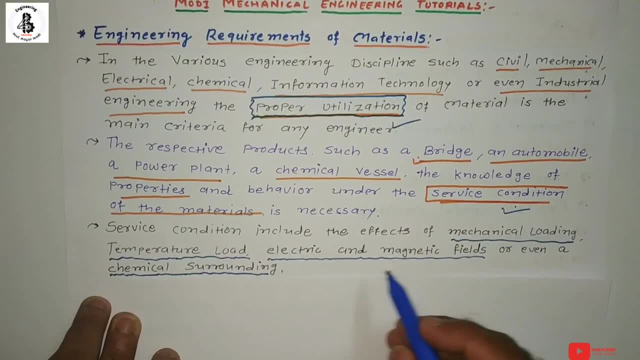 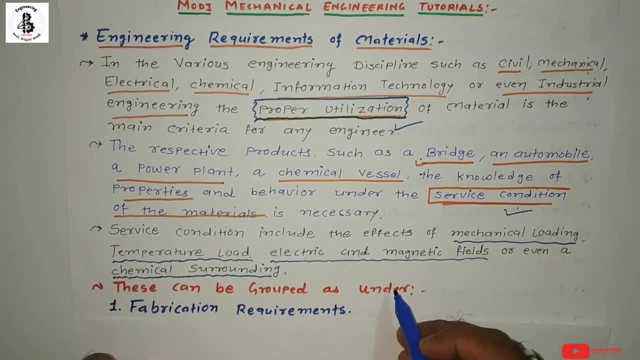 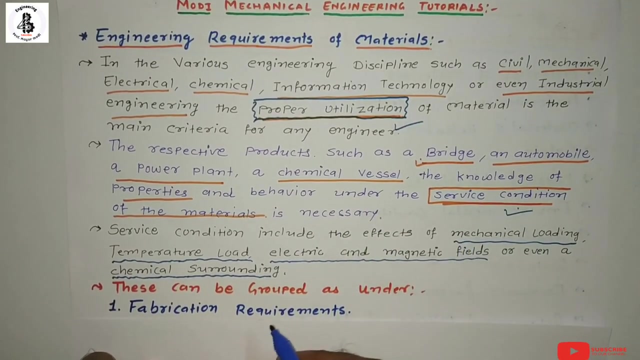 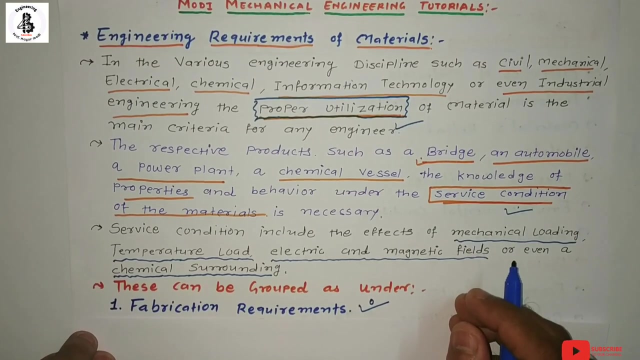 service conditions and the environment effect. So this can be grouped as under: So first of all you have to work on that material which will be having a proper utilization Under the loading conditions. Then the first that will be the fabrication require minds. So selected material, it will be easily fabricated. 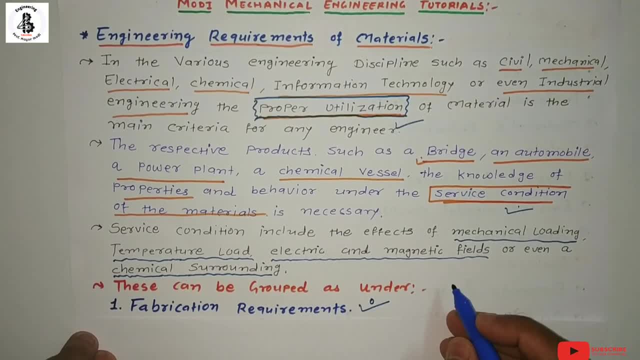 from the raw material to finish product. So which our dannen manufacturing process is going to be use. That will be having a large time Step's. I'm not there any idea if there's any material Water supply is done the round world war air. 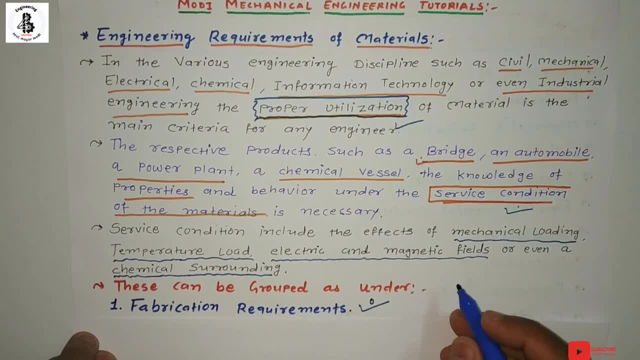 which means the method of supporting of the bottom milliinspires We need than heat, получosing the temperature, taking care that theolyst method is working well. So whatever hace engine meetings And less cost for developing such kind of components which will be used, or you can say proper use- into the service conditions. So that will be the first requirement, fabrication requirement. So so many fabrication process are there. 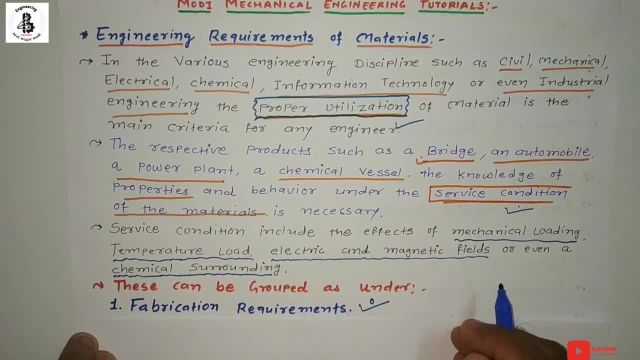 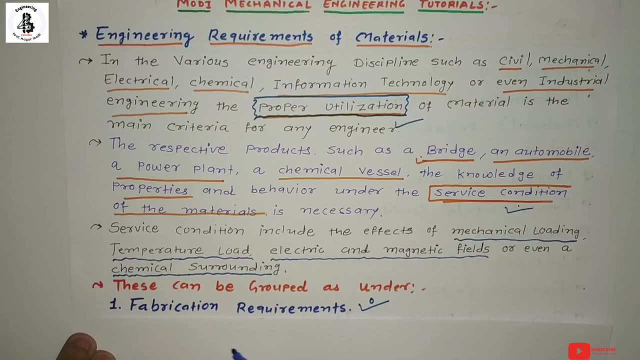 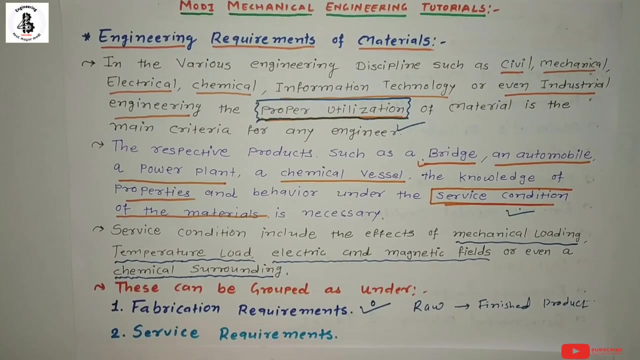 So basically, metal cutting, metal joining, castings, powder metallurgy- So these all are the feasible processes- is available. So by this process you will converting your raw material into the finished product Service requirements. So by the utilization of such kind of raw materials for developing the finished products into the proper utilizations, as well as the under the loading conditions. 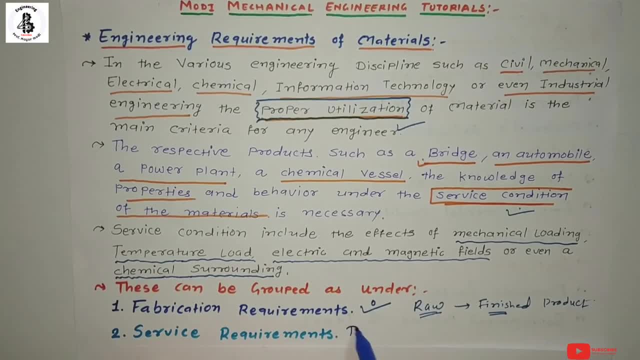 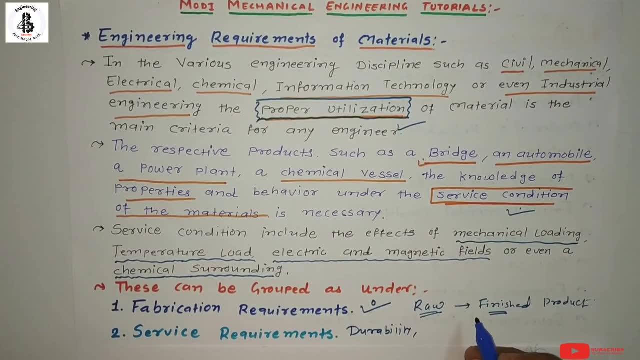 it will be having a good service, or you can say good durability and flexibility, then and then it will be having a hundred percent satisfaction for the customers. so it will be having a good service requirements. so it will be having a high productivity as well as the hundred percent.